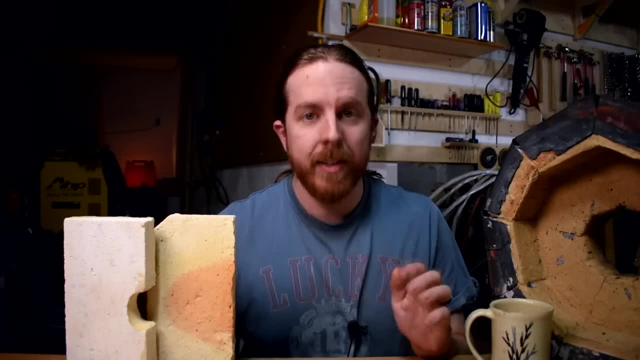 you can use it for so many things. It is just unbelievable how useful they are Like. imagine if you're single and you got to make your own food. It's like a microwave and a toaster oven together, but it can go to 2300 degrees. 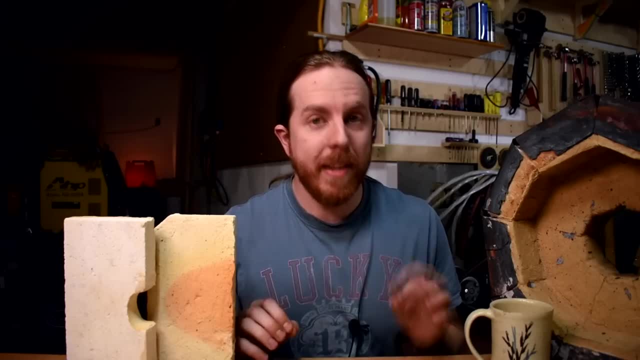 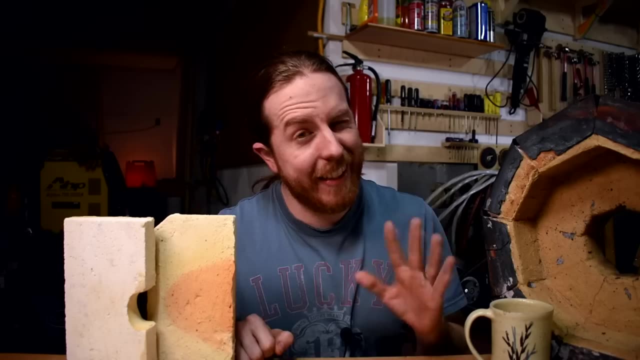 It's, it's at least that's all the hotter I've had mine up to It's. it's crazy. Just build one, please. Problem number one: I built this oven from scratch, so it's a bit it's kind of rickety. 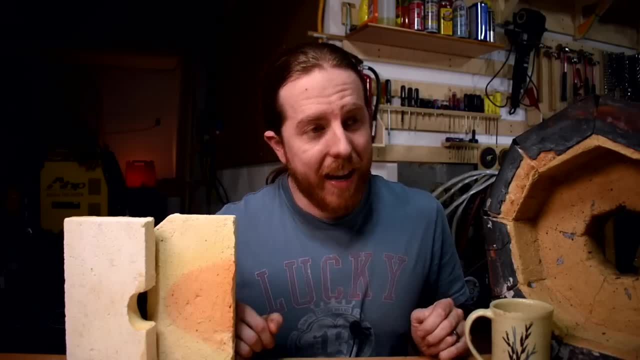 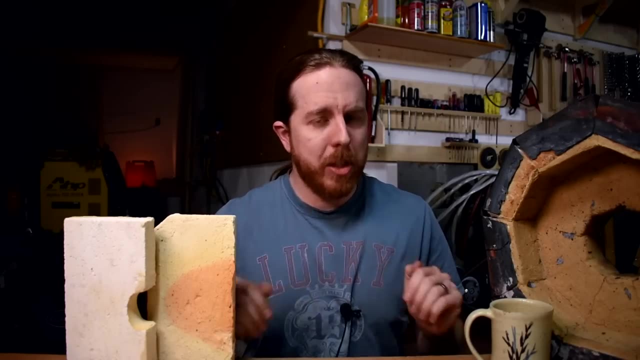 Problem number two: uh, these, these bricks, they're not very tough and I'm asking them, especially the lid, the, the bricks for the door on the top- I'm asking them to handle a lot of stress and they're doing a good job, Admirable job, except for problem number three. Problem 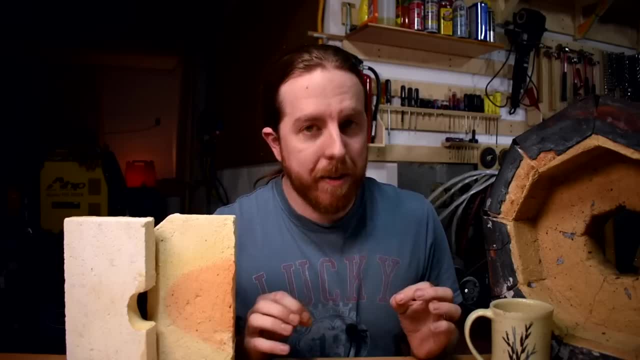 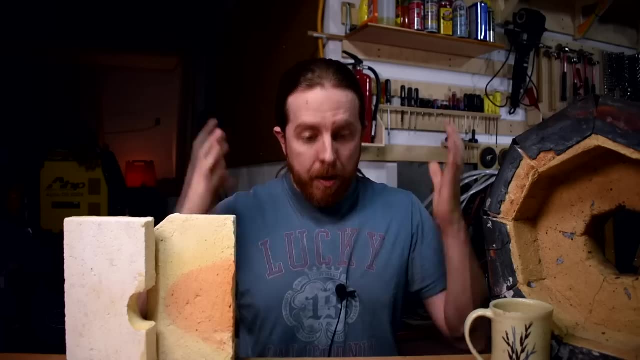 three is one I've never heard talked about outside of, like some pottery circles And and not just not the, not the kilns you buy, I'm talking the gigantic ones you have to design and build in place, Like the ones you got to walk inside to get to your stuff. You know they have. 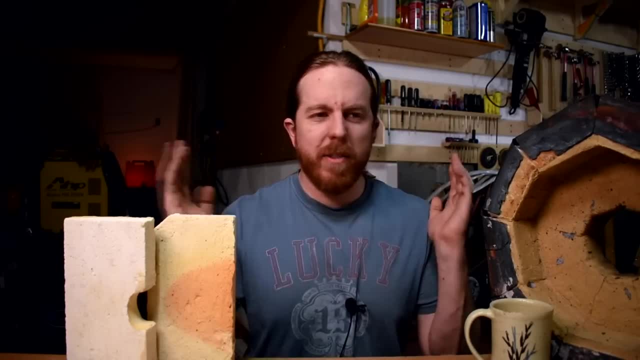 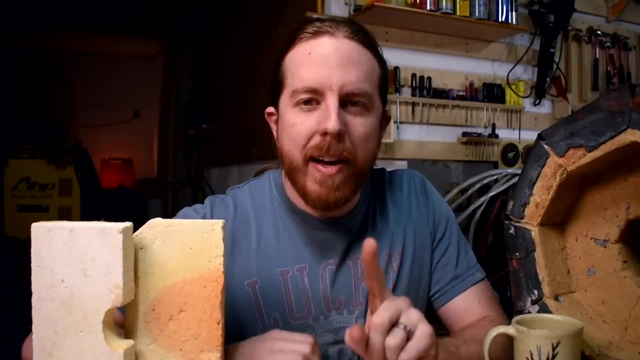 these huge, huge doorways and they fire these things sometimes in well over 2000 degrees, 2300 degrees, for like a week straight. So we're talking a lot of hours on these things. As an aside, I find people get hooked on like one craft you know, like they're only a blacksmith or they 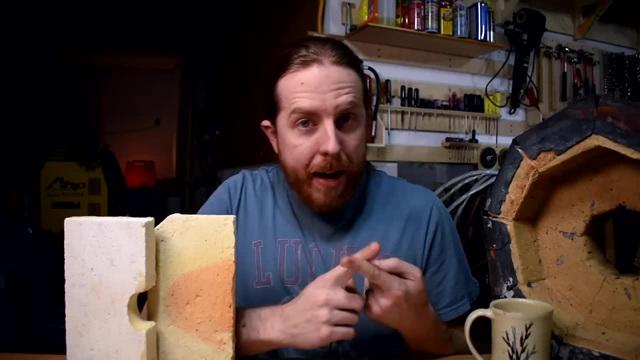 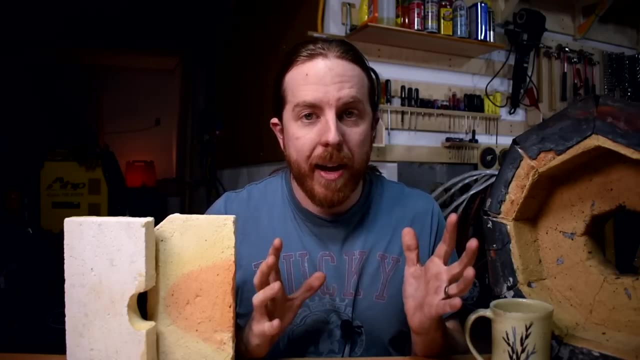 only do metal casting or something. You, you, you gotta get out of that habit. Potters, blacksmiths, metal casters, uh, glass blowers, a bunch of other people use things like a box or something that gets super hot to to do their craft. Get together, compare notes. It might be enlightening, Who knows? 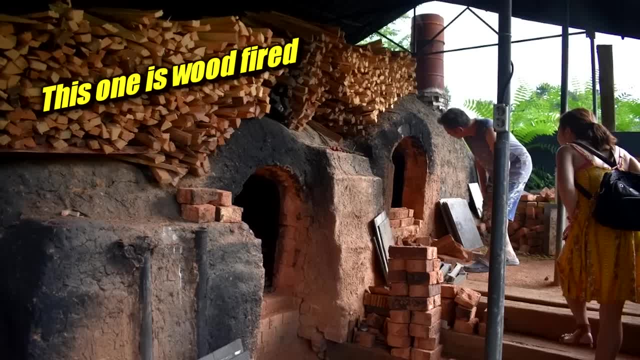 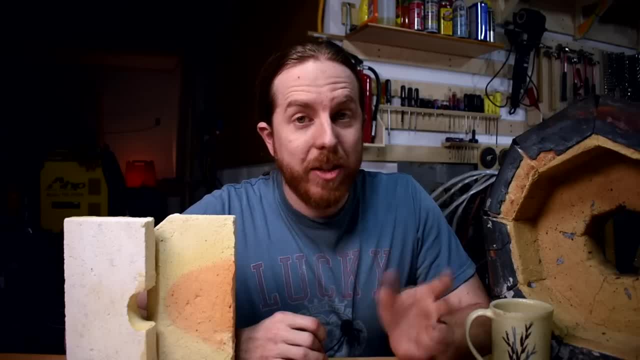 Just food for thought, Uh, but anyways, these giant kilns are usually reduction kilns and you don't want air leaking in, Okay, You don't want any air getting in where you don't want it to get in, And you've got to be able to get the door open when you've got to get your stuff out of there. So 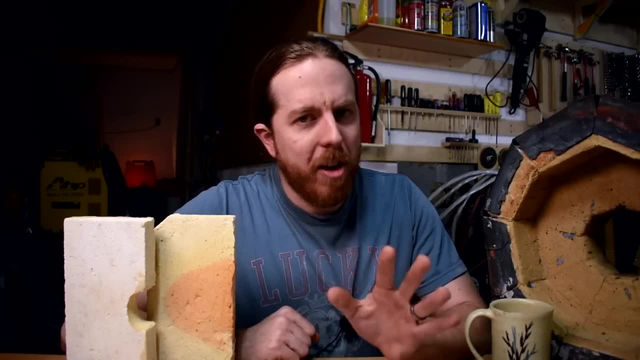 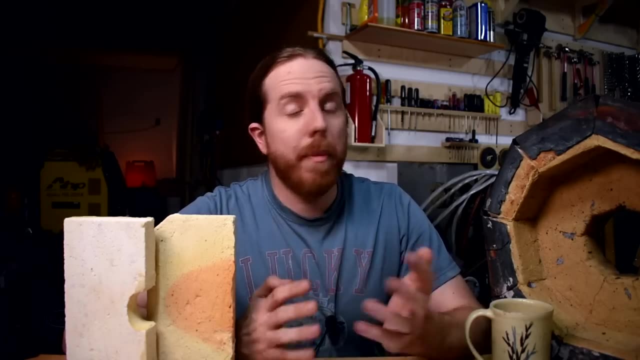 what do they do? Well, they generally take these nice soft bricks and also the hard ones and cut them to perfectly fit inside the opening, No gaps. But the problem occurs after like a couple, a few firings, And at this point it's about like a thousand hours over 2000 degrees. Uh, so it takes. 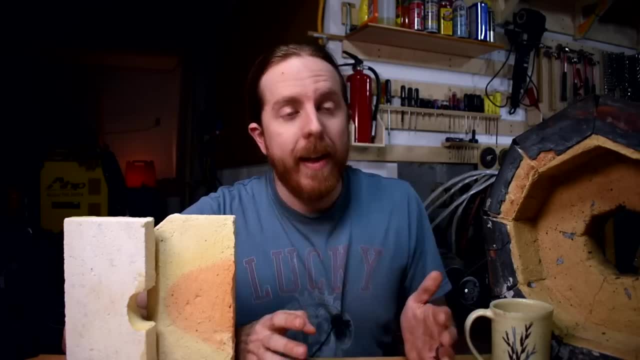 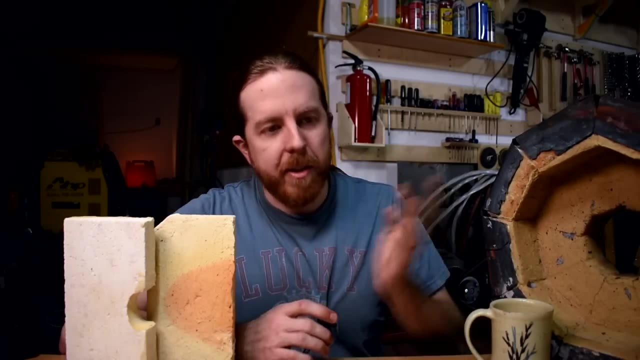 a while. Uh, but those bricks, they suddenly they don't fit very good anymore And you gotta start shimming them. You gotta like cut like little thin ones so you can slide them in the openings. They shrink basically. They shrink ever so slightly. They also like smear clay over the thing. 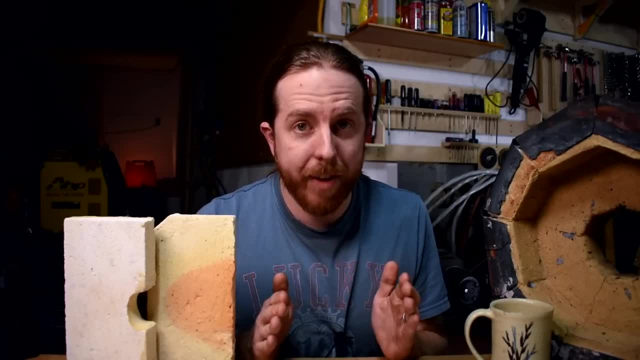 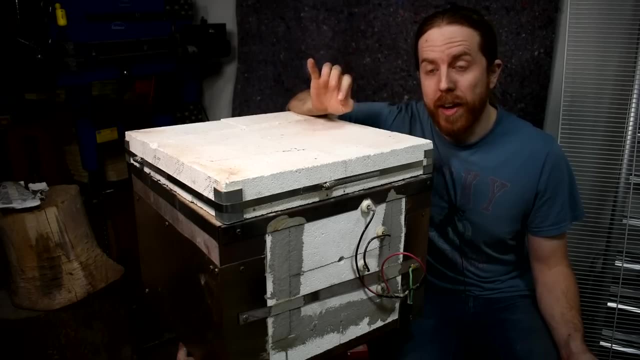 so it plugs all the gaps And, anyway, forget it. The shrinkage is the problem I'm having right now. I had heard about this problem from a documentary about, I think, English potter, Phil Rogers, And I planned for it. So this, this oven that I built. 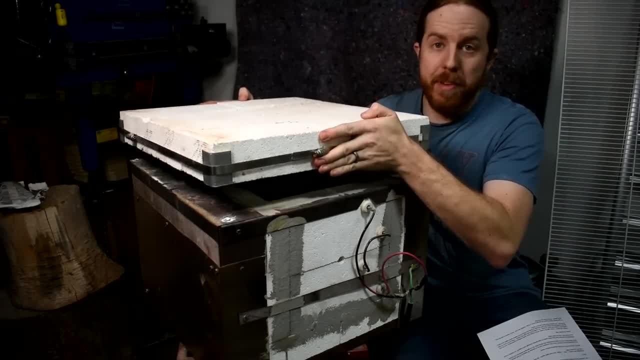 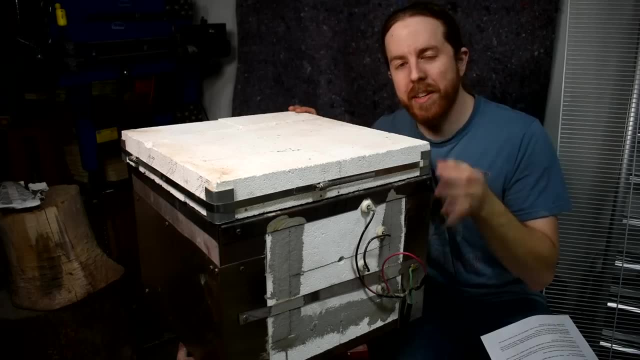 has a removable top. This is the door. See it just, it just lifts up. There's no hinge or anything, And it's just eight bricks, uh, held together with a band clamp. Some some angle here for the corners When they shrink. they're just shrinking a tiny, tiny, tiny bit, But you know, over time 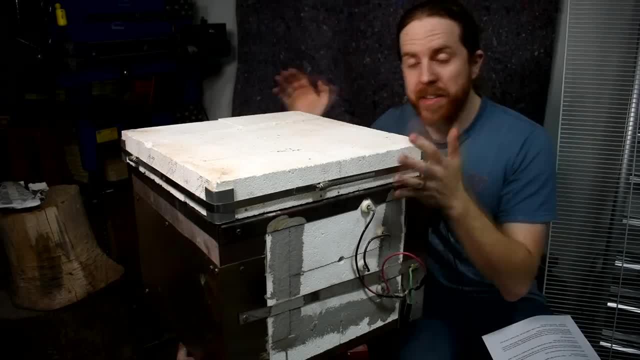 it's enough to build up to be a problem. I figured, as that happens, I could just keep it tight and put it in the middle Right. Well, it didn't. The lid just fell in here in the middle, You can see. 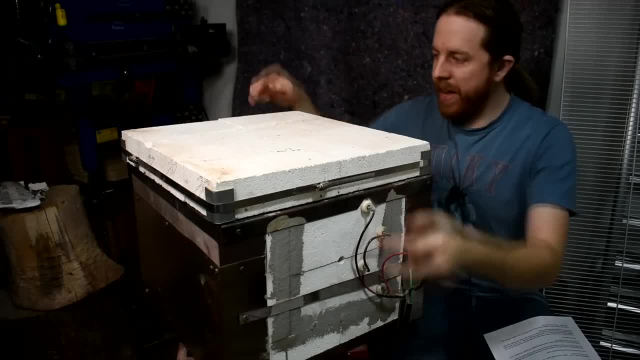 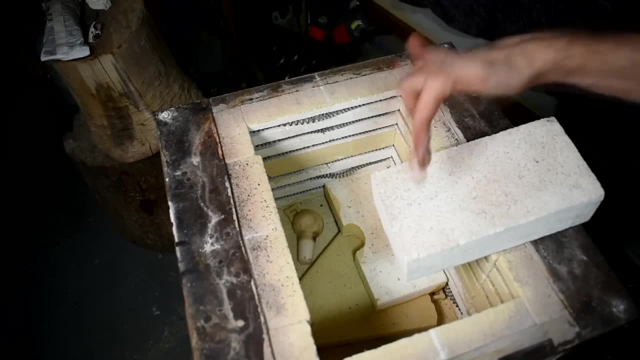 it. It really didn't matter how tightened I made this thing. It tightened up nice. The middle still fell in, Okay. So look at this thing from up here. When the bricks go on, they kind of sit like this right: Only part of it is covering the opening, And in here is the hot box, Not a hot box, No. 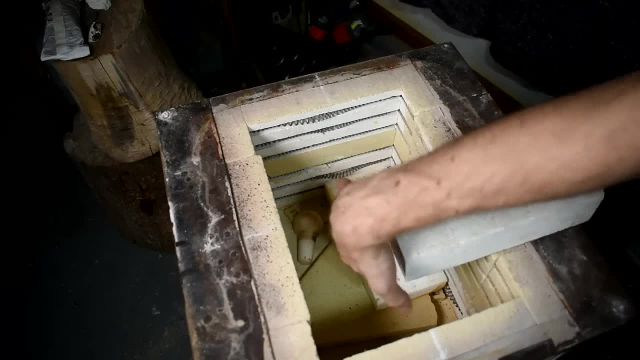 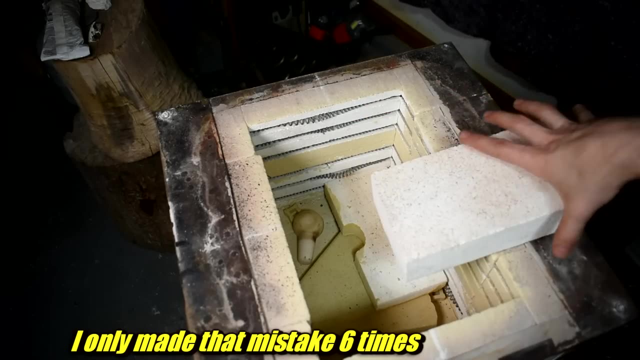 that's wrong word, wrong terminology. So this side of the brick, you know, gets exposed to all the burning heat and out here it stays relatively cool. I mean don't touch it or anything, but it's not glowing white out here. So that means 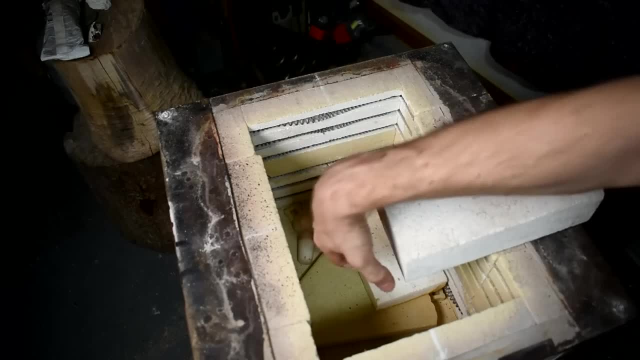 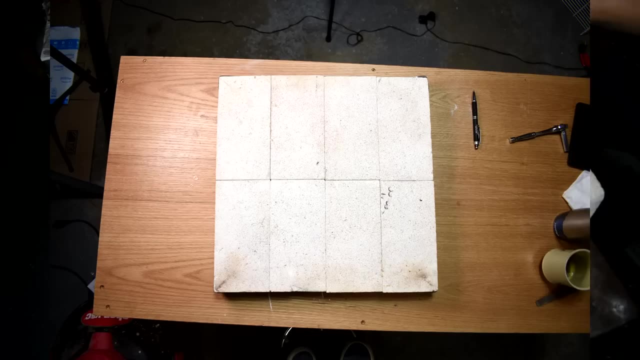 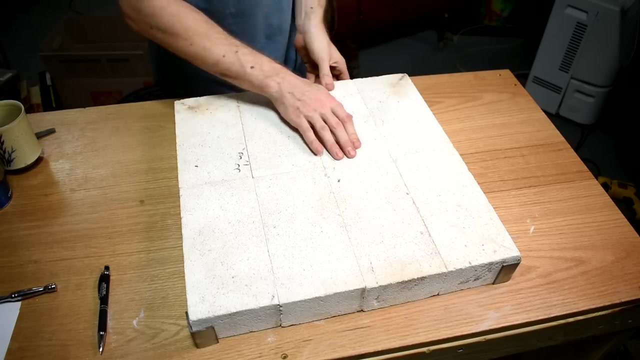 is the inside here has shrunk a little bit, just a little bit, and out here hasn't, And this happens, like all, all the way around. So if I tighten that that band clamp, it just tightens along the perimeter And this inside part is still all loosey goosey. Okay, I can confirm this. 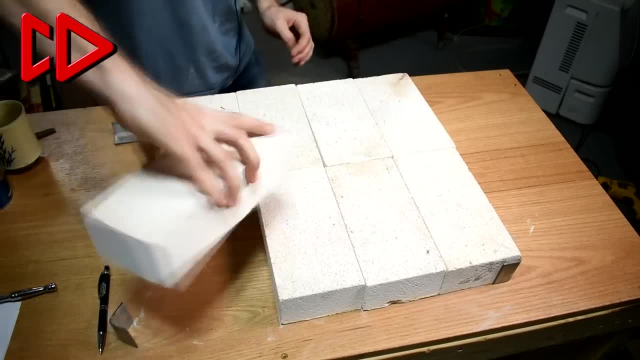 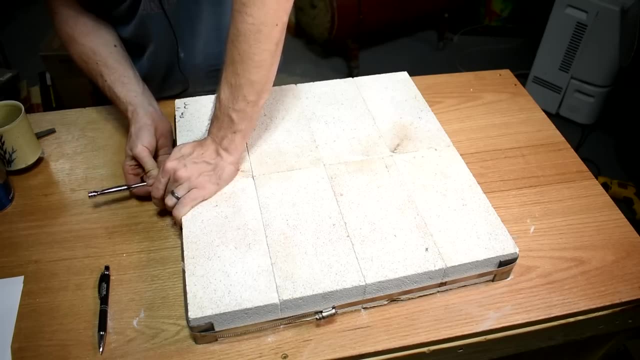 by flipping the bricks around, So the loose parts on the outside, the tight parts in the middle, and re tightening the clamp and see what happens. Okay, Retighten this band And let's see how it works. I should be able to just pick it up by the. 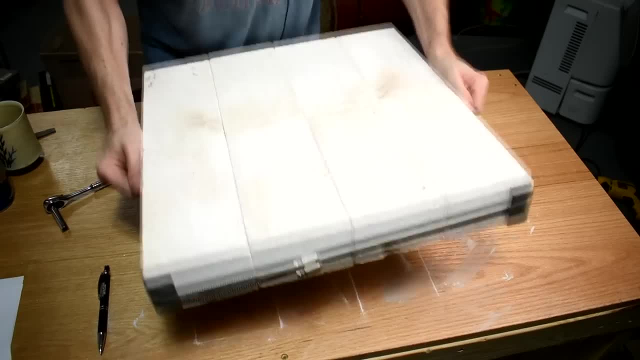 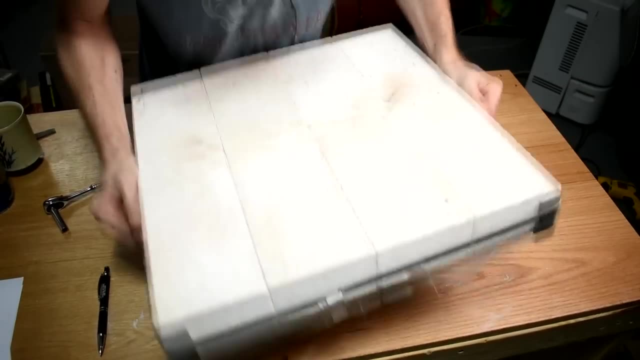 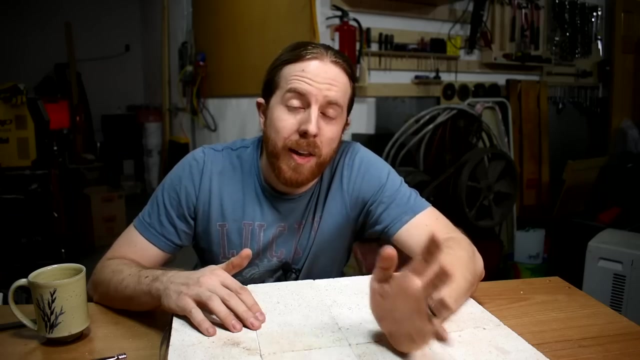 by the clamp and then them not like collapse. Hey, look at that, It's tight again. Earthquake test. They're not falling down, Bingo, Okay. So all I've done is kick the can down the road a little bit. 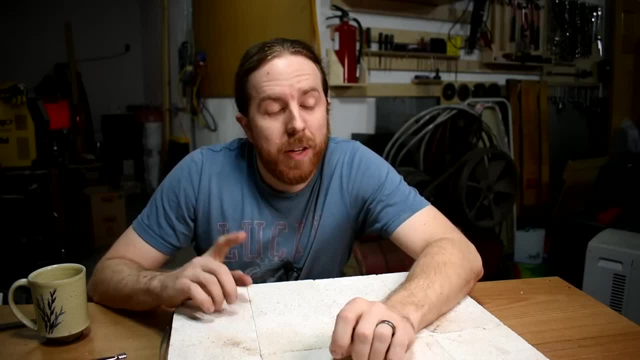 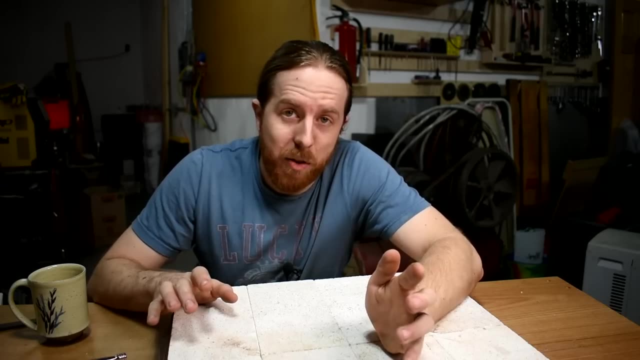 This is all just going to happen again. How do I prevent it? Well, the foundry furnace lid doesn't have this problem for a couple of weeks. So I'm going to go ahead and do a couple of reasons which we'll get into later, but I'm too lazy to redesign this whole thing from scratch. 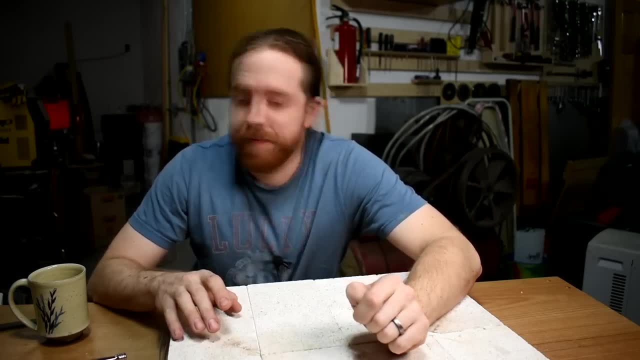 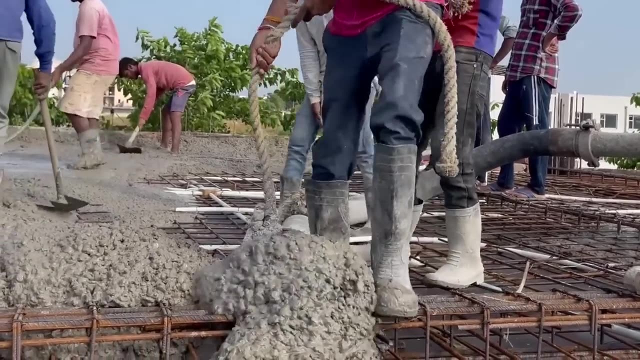 right now. So I'm going to reinforce the bricks. Reinforced concrete has long rebar poles to add tensile strength and support, So clearly I need to do that here. Uh, but not with rebar. This is steel Now. I never get the inside of this thing quite up to steel melting temperature. 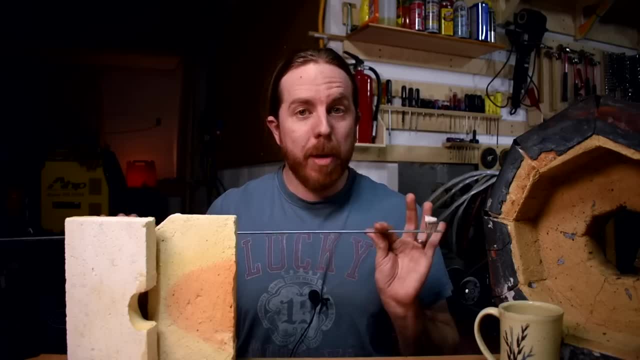 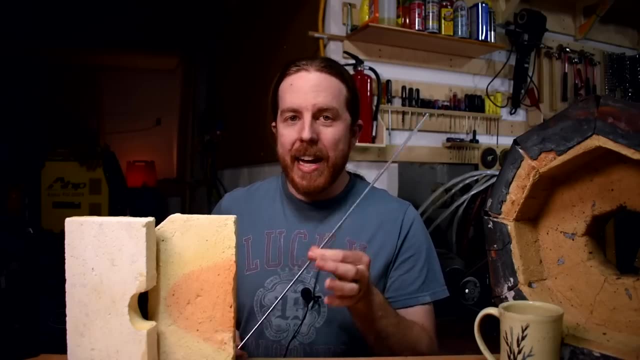 definitely hot enough to weaken steel. but I'm not putting this inside, I'm going to put this through the bricks. They don't have to hold all the way to this thing. They just have to have enough strength so that, if the top were to start bending, this can kind of hold it in place. 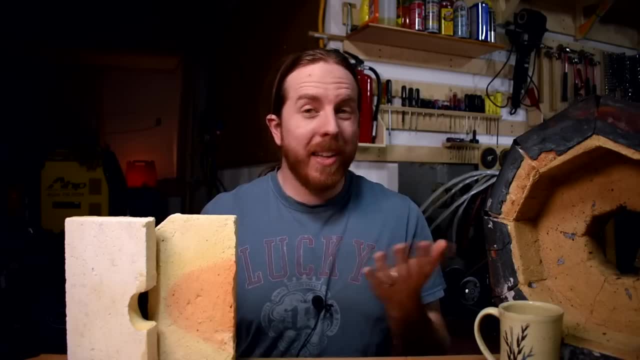 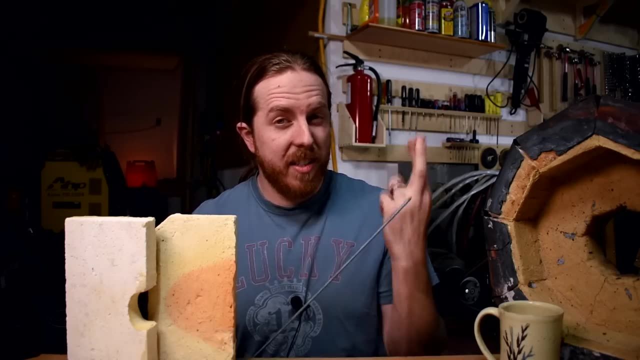 I am leaving the band clamp in place, I'm keeping it tight and I'm only going to lift the lid, like when the thing is turned off anyway, or at least not that hot. So this, this should be good enough, Fingers crossed, If not, we'll definitely know soon- So to get these rods through the bricks. 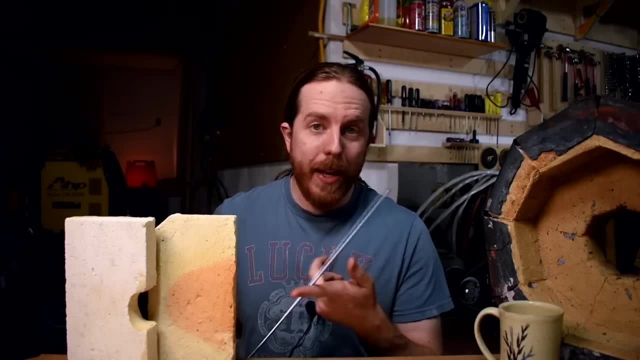 I'm going to have to bore a hole and I'm going to use the rod to do it, but it needs a drill bit end, so to speak. So here's how you do that, Using like a grinder a file or something. give it a. 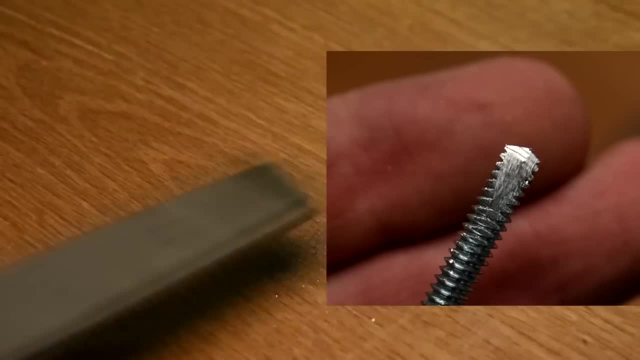 bend, Then I like adjust it to let it a slight point in the middle. This is kind of like a drill bit end. you know It's it's a lot worse, but the brick is pretty soft, It should work out okay. 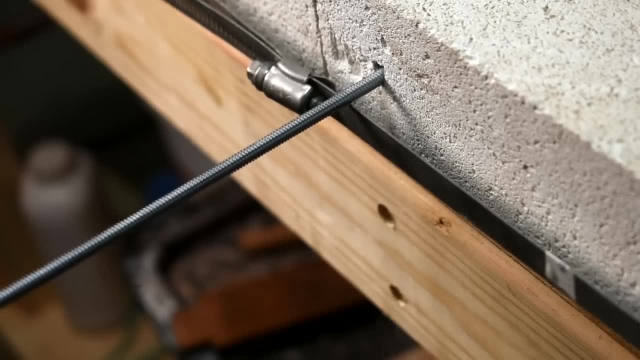 Fingers crossed. I'm going to run it through the sides like so. I mean, if I had a big drill press that I was sure was straight, I would use that. Since I don't, I'm going to hope I can use the. 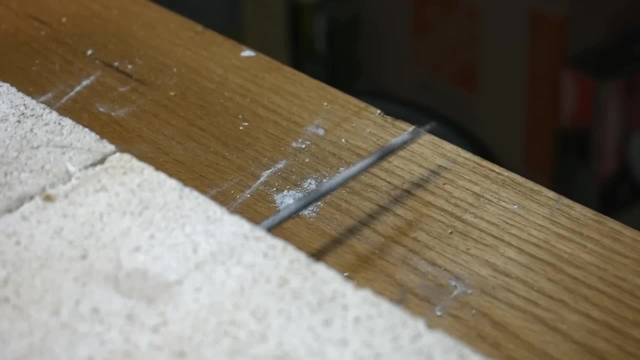 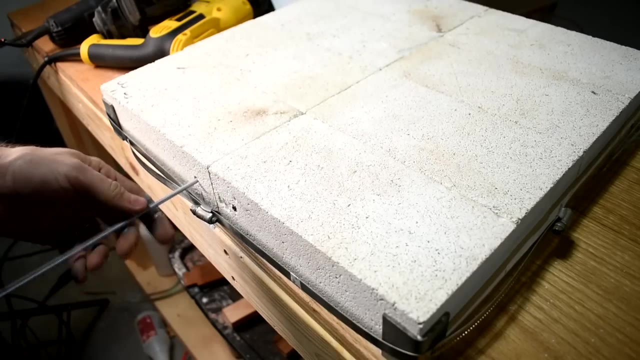 force or whatever, and get it through straight with the normal handheld drill, Then cut the end off with an angle grinder. It just so happens this threaded rod was exactly twice the width of the lid, so I don't even need to get another threaded rod. 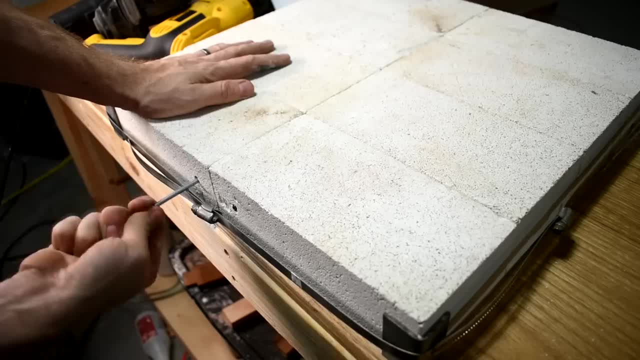 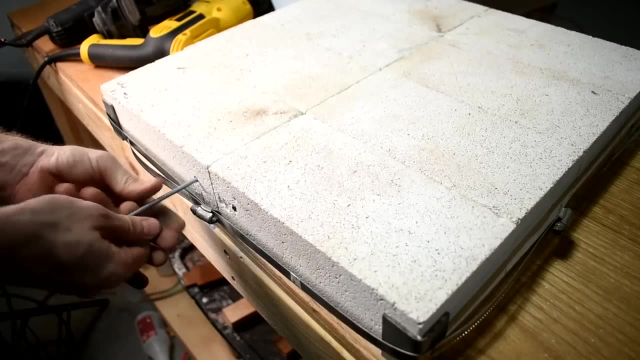 Okay, the hole is a little tight here, you know, on account of it being drilled by this rod. Not a lot of extra space. I suppose I'll just thread that right in. That was surprisingly easy to do. Kind of shocked. I'm not going to thread a nut on either end. I. 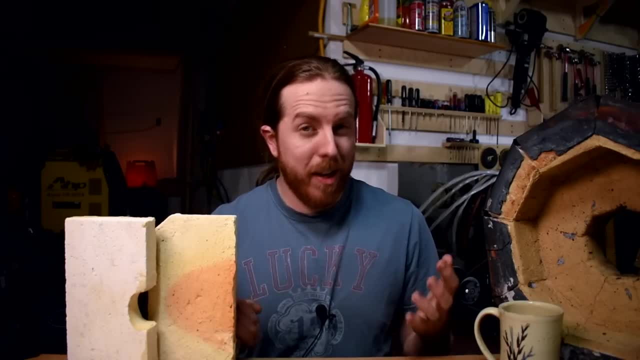 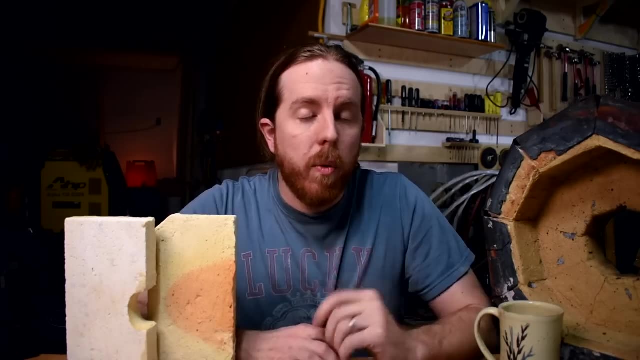 want them to have room for expansion. I also want to be able to like remove them if they do get gross and like shove something else in there. I don't know, maybe it'll get tungsten in the future, but hopefully it's good enough for at least a few heat cycles. So what can you do in the future to 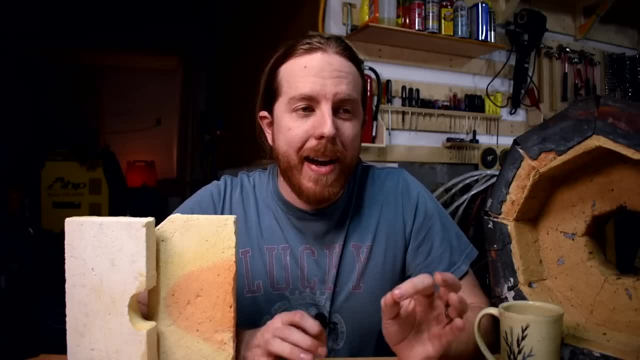 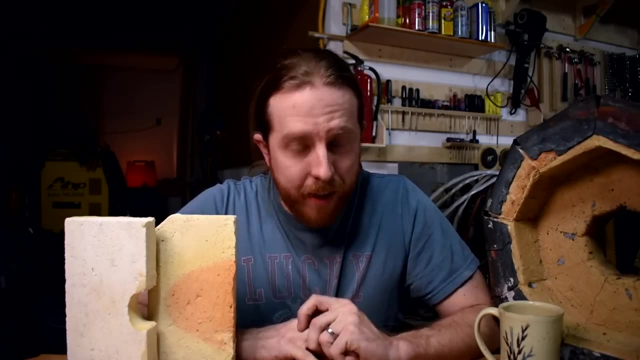 prevent needing to do this on yourself Because, like what I just did, let's be honest, it's not ideal, It's a bodge job. But if you're designing it from scratch, take a look at other fire brick structures. The roof on many kilns aren't flat, They're like 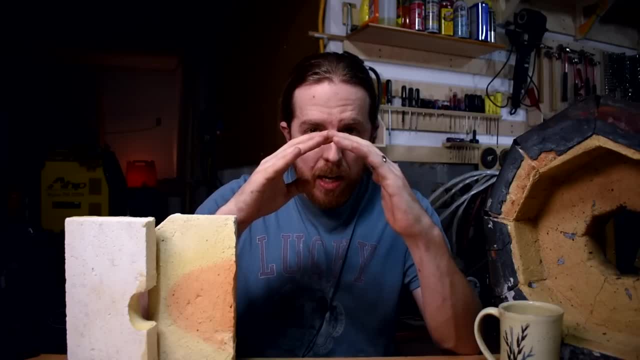 arched. You know, if those arches, if the bricks and the arch start to shrink, it's just going to lower the arch slightly and they're all going to be tight again. It's brilliance of an arch, You know, and the amount the bricks shrink it's very tiny. 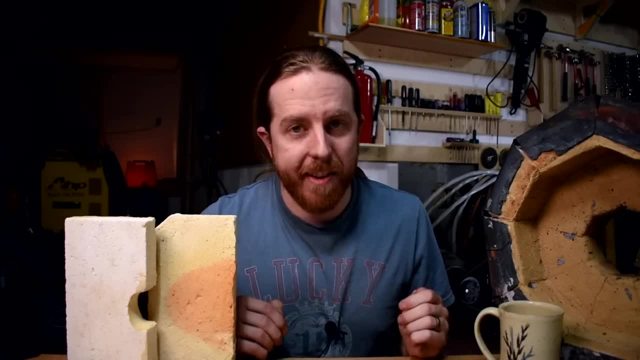 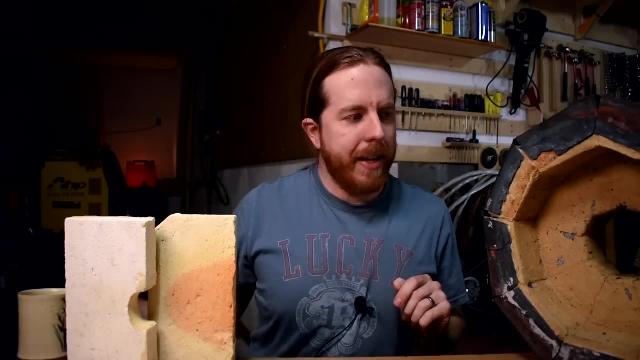 so you're not even going to notice, But the structure will automatically fix itself. It's really cool. There's also, like the furnace, foundry lid, like this one. So with these ones, it's getting dust in my teeth With this thing. you might think like this metal part is what's. 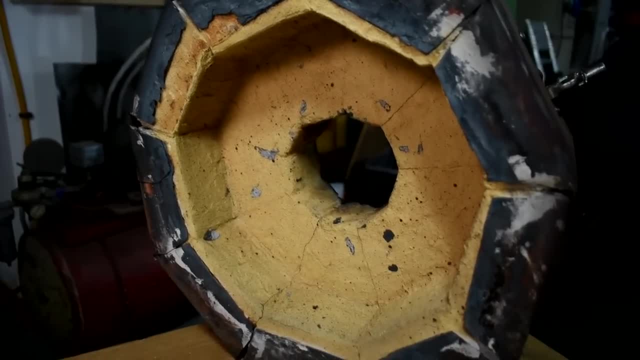 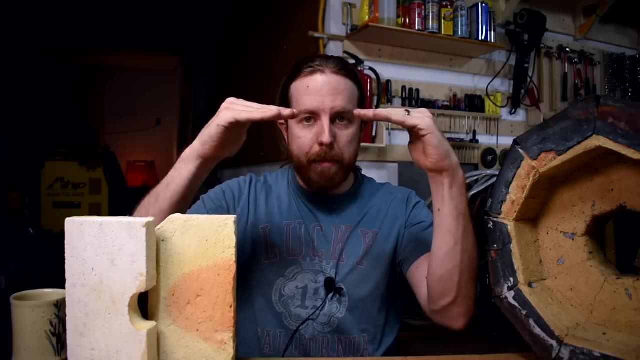 holding it together and it kind of does and it's got this flange holding them up. But really the bricks on the inside here they're shaped like a wedge, So if any of them- and they're like held up on the edges here, so if any of them were to tip, they would tip. 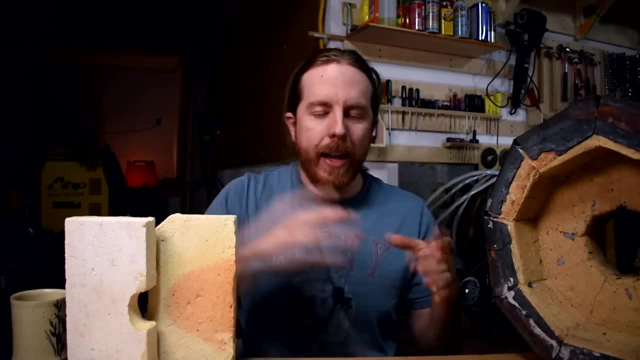 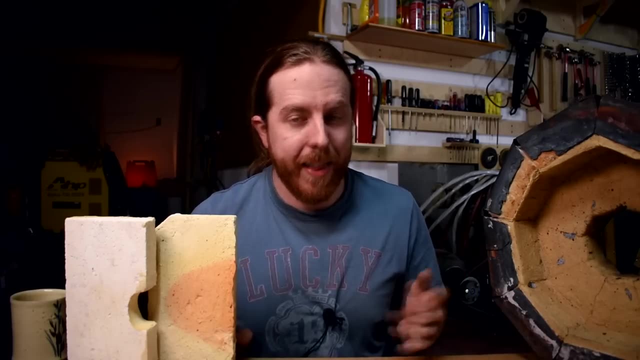 forward towards each other, And because the top is wedged, I know there's a hole in it, but because the top is wedged, when they move forward they push together, kind of like a Roman arch- Not as well, kind of a screwy version of that, but it's a similar idea. 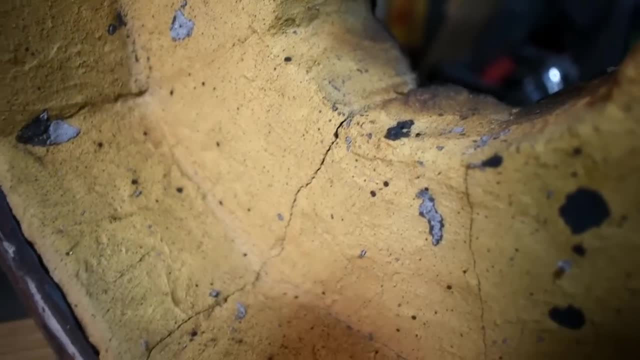 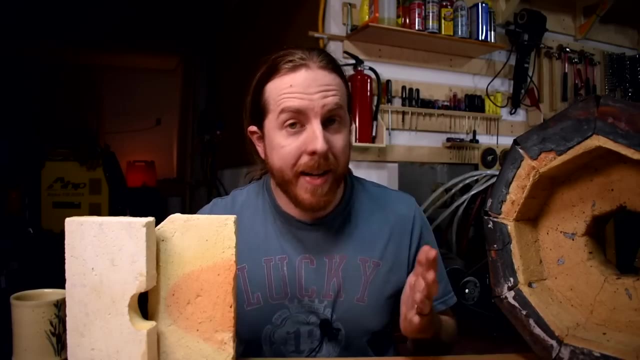 So this: although there's big cracks in it from the lid, you know heat cycling and shrinking a little bit- it's still holding together. Also, I've been patching it with Satanite. that helps, You know, like there's a reason. 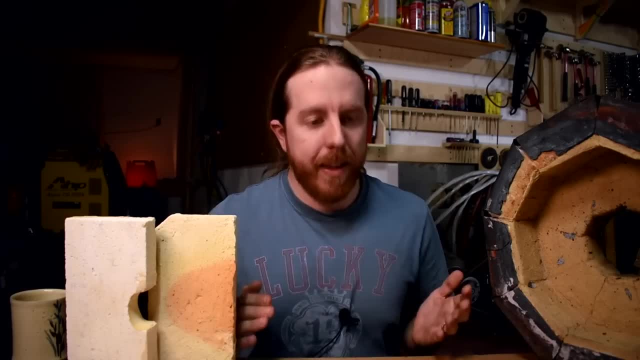 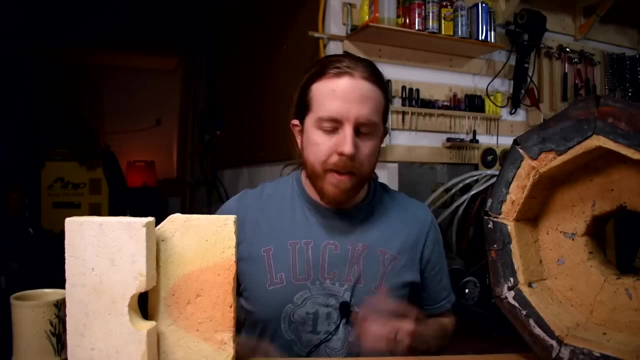 those Roman buildings have been standing up so long and it's not the aliens who didn't build them, It's because the design is just smart. Romans were pretty smart when it came to building stuff, So like if that band clamp, like squeezed in on all the edges and not just the corners. 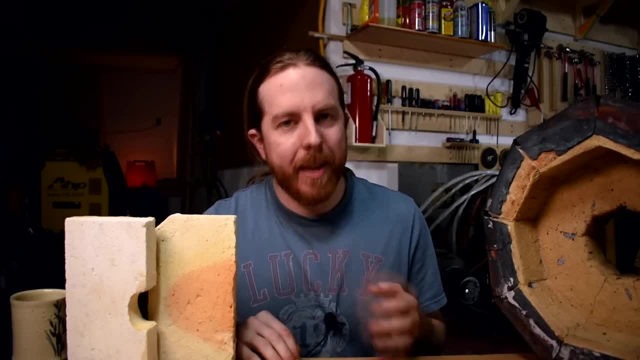 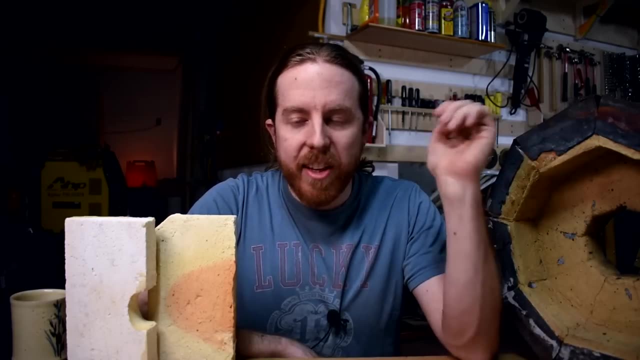 it would probably be similar to this, But they don't because I didn't engineer it very well. To be honest, Another method you can do: just make the lid, like, seal it all up, Put the door on the front, Like a lot of the ovens you buy, the fronts open up. It's never a problem. They. 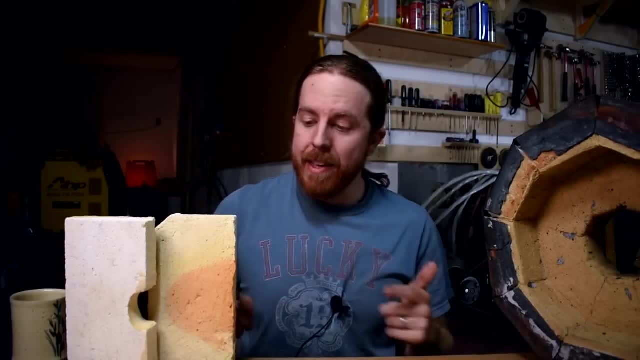 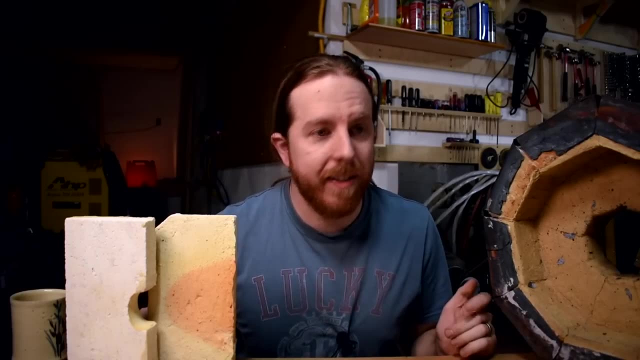 also tend to be a little smaller. One thing you can do: you can actually get these bricks in larger pieces. You can get a full like foot and a half by foot and a half square of it. They just cut it this shape because it sells better. You know they can move a lot of them. 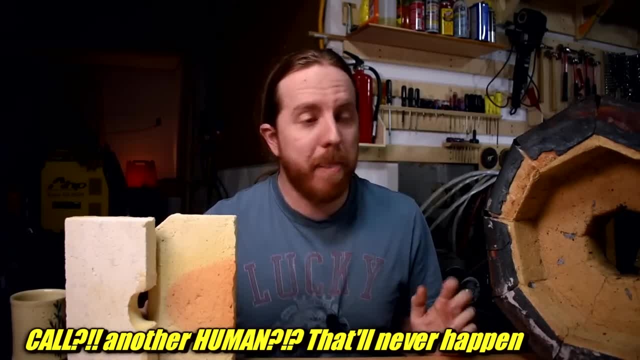 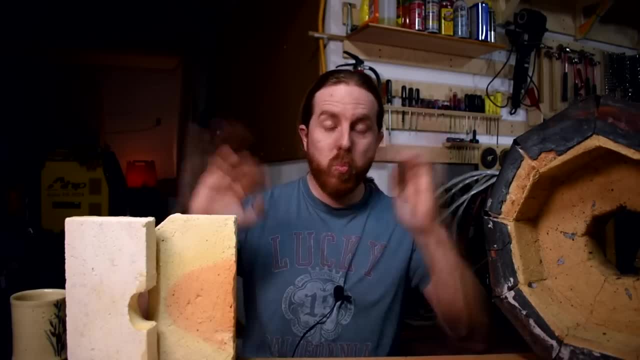 But if you call them up on the phone, you can get a single piece as big as you want. Why didn't I just do that? Huh, Whatever It's fixed, Ready to burn out some PLA or whatever. I'm making this stuff up as I go.